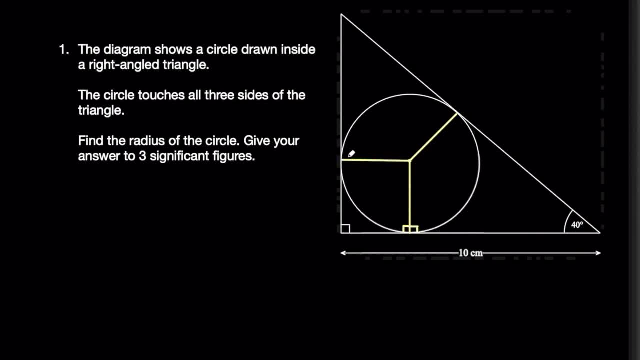 is going to meet this line of the triangle at 90 degrees. Same for this one and same for this one up here. Okay, the other circle theorem you're going to need is that tangents to a point are the same length. So these tangents, which are also the side lengths of the triangle, from the point where 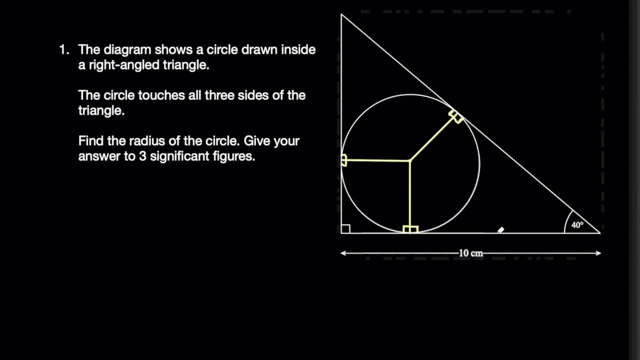 they touch the circle to the point where the two lines meet, those lines are equal length And actually, if you go all around the triangle, all of these lines are tangents to a point. So they're all going to be equal in length to each other, And these ones down here will also be the same. 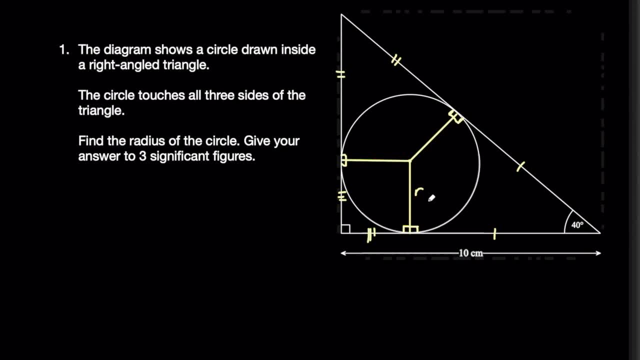 same length. Let's also label the radius of the circle R And you might notice another shape in here. So we've got the triangle, the circle. Can you see another very familiar shape in this diagram? Well, now that we've drawn in these 90 degree angles, 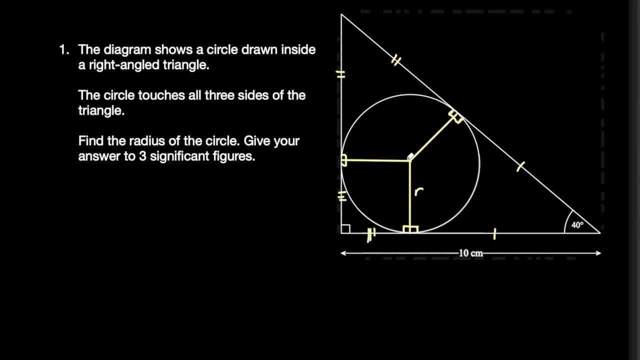 well, if you've got three 90 degree angles, the other angle must be 90 degrees And we have a square in here. That means that all of these sides will be equal to the length, the radius of the triangle. So we can label this one over here R as well, And we're almost done setting this up. We. 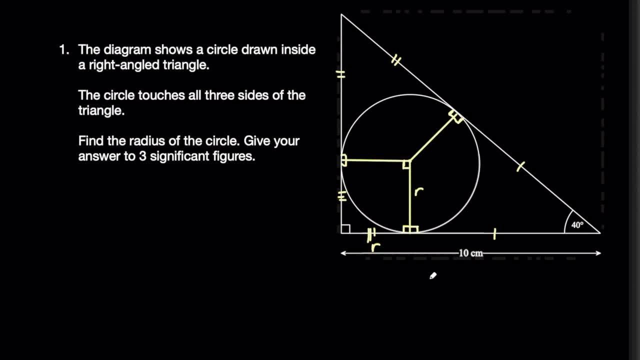 just need to draw in one more line. Where do you think that line's going to go? That's right. it's going to go from the center of the circle to the angle over here. Now that line bisects that angle, because these two triangles must be congruent, right? They have two sides that are the same. 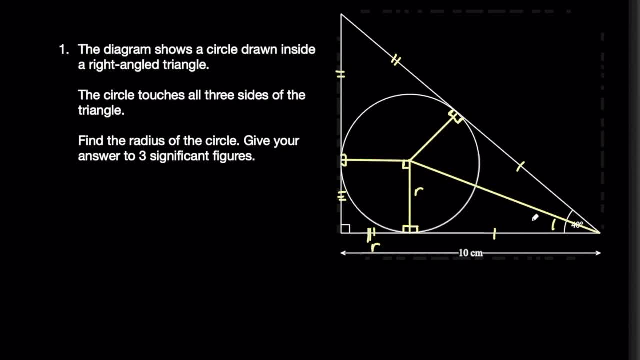 Therefore, these two angles in here are going to be the same. So half of 40 is 20 degrees. Okay, we're going to start to solve this problem. We can go ahead and start to solve it. The first thing I will do is label this length here. I'll call this A. Now I have this right angle triangle in here. 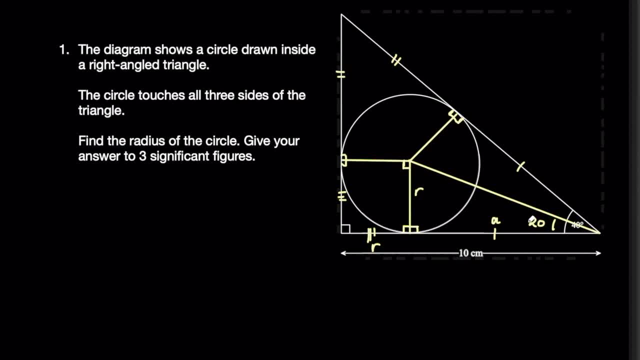 with side length A and side length R, And I have this angle of 20 degrees. Here the trigonometry comes in. So which ratio am I going to use to relate these two sides together? That's going to be the tan ratio, right? The tangent is the opposite side over the adjacent side. So we could firstly say: 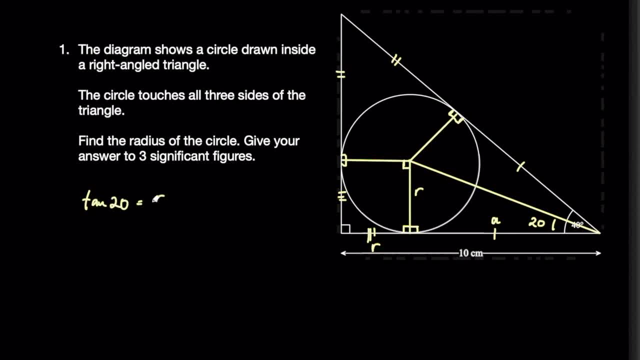 that the tangent or the tan of 20 degrees equals R over A. And then I want to write this in terms of A, And you'll see why in a minute, So I can rearrange this so that A equals R over 10 of 20. 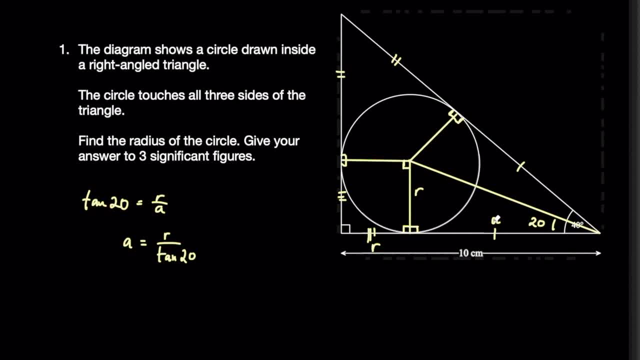 degrees. And now I want you to focus on this long length here. We've said we've labeled this length A and this length R, because we know it's the same length as the radius, because this was a square in here. So if A plus R is 10 centimeters, I also know that A equals R over 10 of 20.. So I can also say: well, let's start off by saying that A plus R equals 10 centimeters. 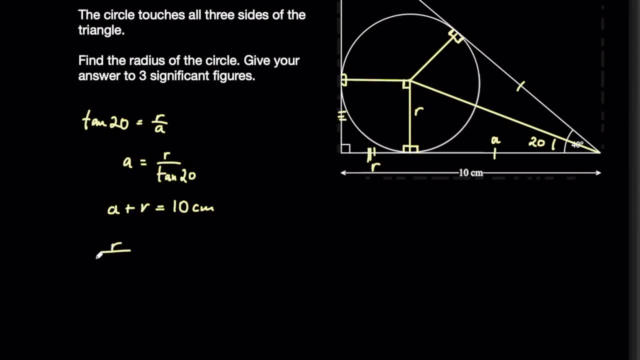 Then substitute this in for A. We can say that R over 10 of 20 plus R equals 10 centimeters. So the first thing I'll do here is find the value for 1 on 10 of 20.. So I can get a coefficient of R. 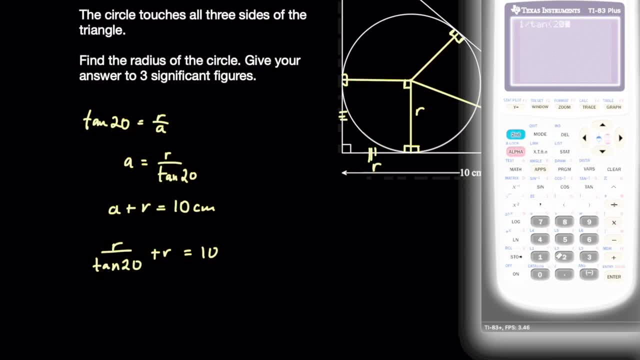 1 on 10 of 20 degrees. Actually, I've got to make sure my calculator is in degrees first. That gives me 2.747 approximately, So this can also be written as: 2.747R plus R equals 10.. If I simplify this, 2.747 plus 1 would be 3.7467.. 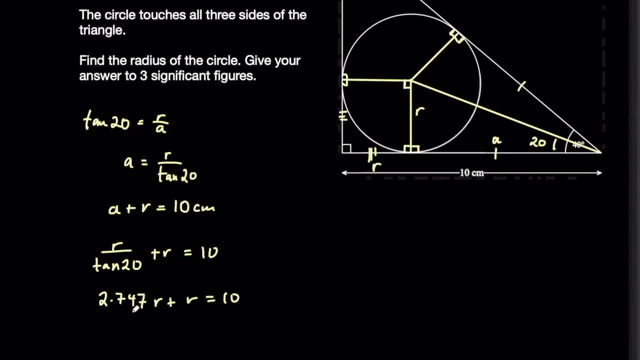 So I can get 2.747. R plus R equals 10.. If I simplify this, 2.747 plus 1 would be 3.747.. so R is going to be 10 divided by 3.747 approximately. I should use approximation. 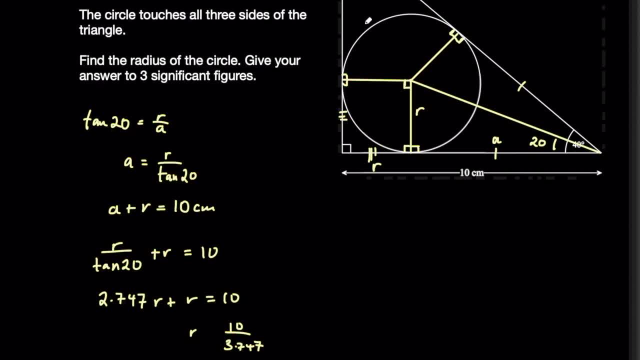 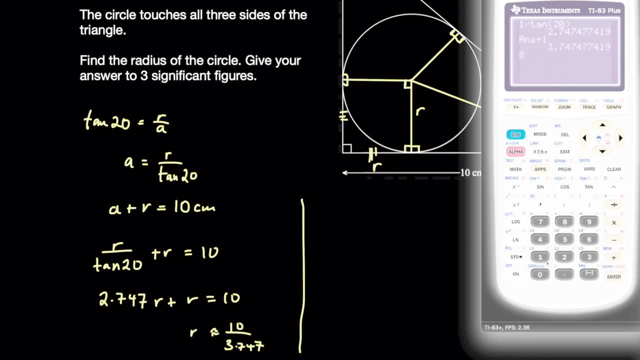 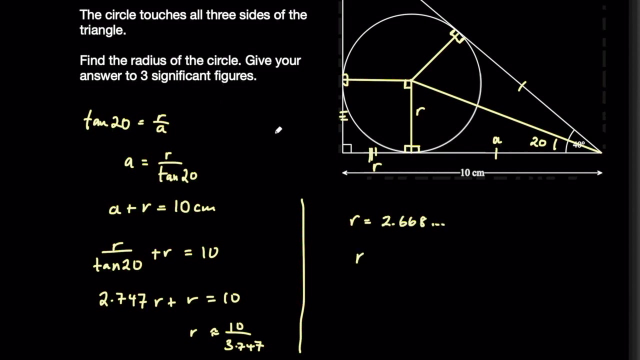 symbols here. Okay, so now I just have to get a value for that. I'll add one to this and then divide 10 by that answer and I get 2.668 approximately. So R is equal to 2.668, and rounding off to three significant figures I would get 2.67 centimetres. Okay, so that. 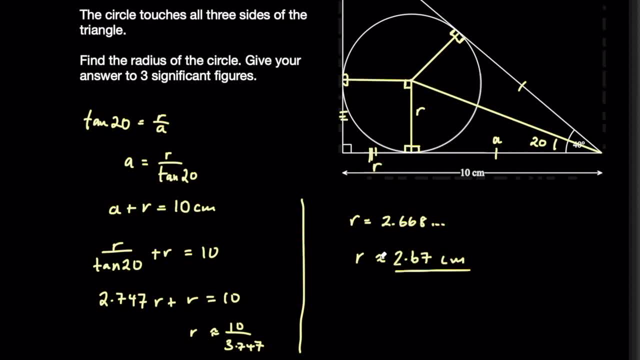 is how, or one way to solve that problem. There are different ways. There is a much longer way to solve that problem. You can set up simultaneous equations by labelling all of these lengths. There's nothing wrong with solving it that way, it just takes a bit more. 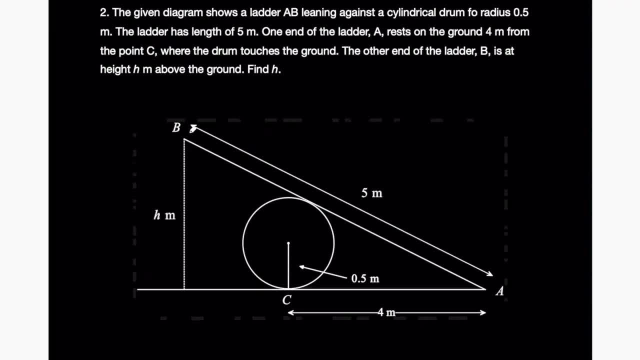 work. Okay, on to the second problem. This question says: the given diagram shows a ladder AB leaning against the cylindrical drum Of, that should say of- I'll fix that in a minute. Of radius, 0.5 metres. The ladder has length, 5 metres. One end of the ladder A rests on the ground 4 metres from the point C, where 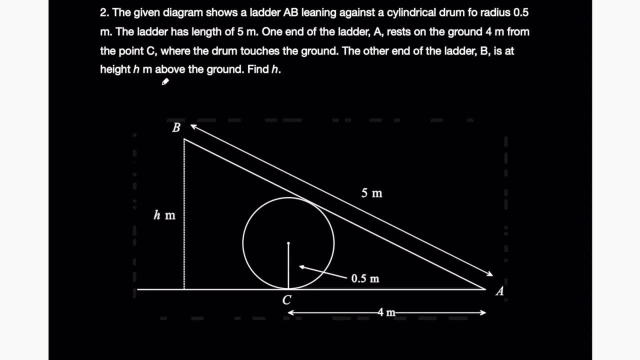 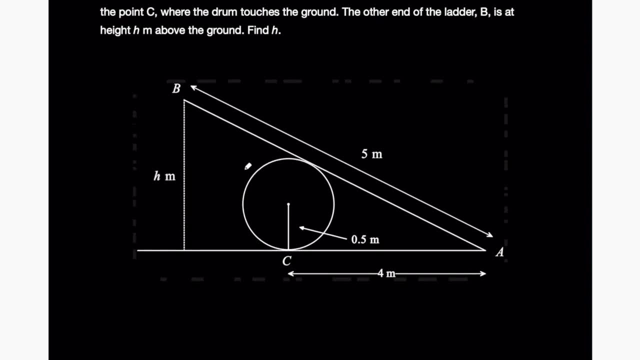 the drum touches the ground. The other end of the ladder B is at height H metres above the ground. find H. So all of that basically just summarises this diagram. We have a ladder, supposedly of 5 metres, leaning against a drum and the radius of the drum is 0.5 metres, and 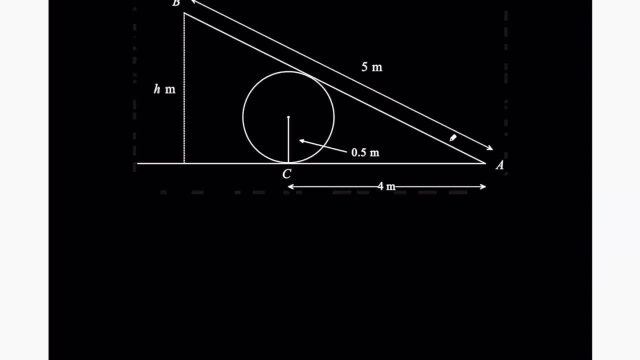 we need to find this length over here. Well, one way you can do this is to focus on finding this angle in here, because once you have that angle, you'll be able to use the sign ratio to find this length. So how can we find this angle? Well, we just hinted. 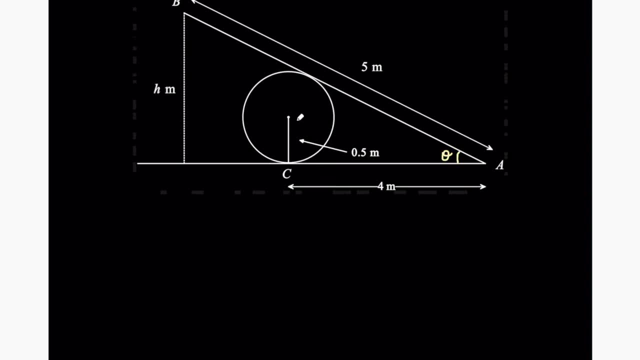 at it in the last problem. actually, If we draw a line in from the centre of the circle to this angle, we know it bisects that angle, So I might just re-label this. I'll label the smaller angle theta and then the large one can be 2 theta. Well, I can find this angle. 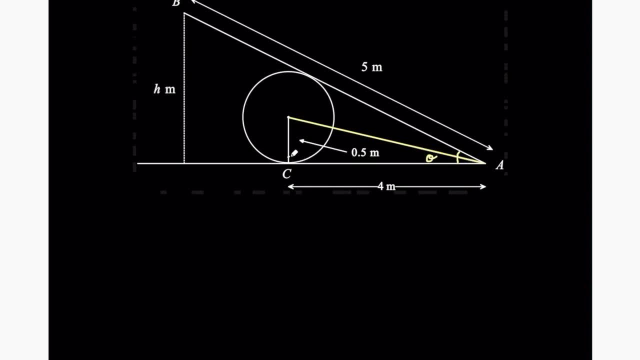 because I have two lengths of this right angle triangle. I know it's a right angle triangle Again because this is the radius meeting the tangent at 90 degrees. So I can use the tan ratio again. Tan of theta equals the opposite side over the adjacent side and this allows. 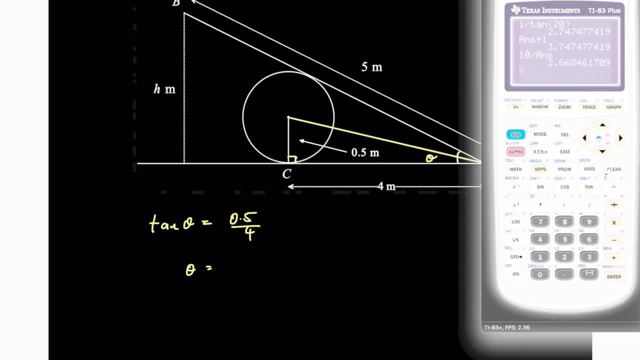 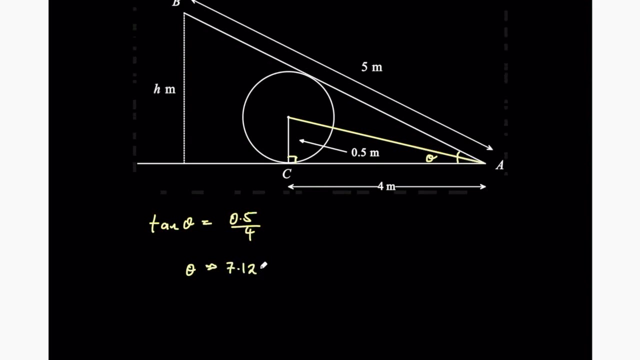 me to find theta by using arctan or inverse tan. So I can do the inverse tan of 0.5 on 4 and I get 7.125, approximately, Approximately 7.125.. So then 2 theta is going to be double this. So now I have that angle in here. the 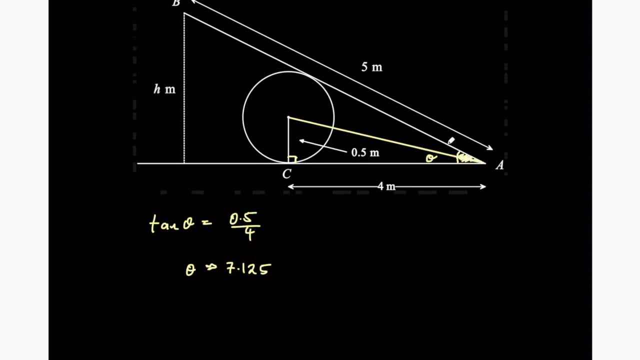 whole angle of BAC and I can say that sin of 2 theta is going to be the opposite side over the hypotenuse. And again this must be a right angle triangle because this is the perpendicular height from the ground to B, So sin of 2 theta is going to be the opposite. 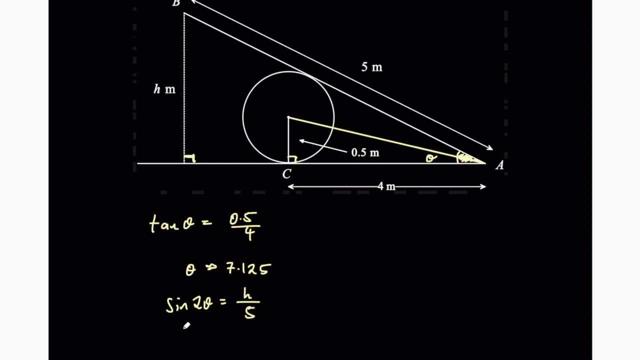 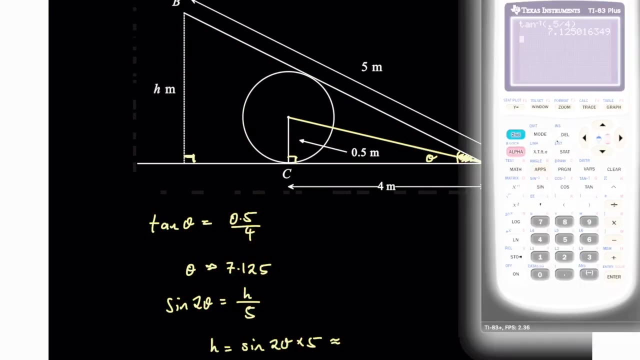 side. So sin of 2 theta is going to be the opposite side over the hypotenuse. And then again we can solve for h because we have 2 theta. So h is going to equal the sin of 2 theta multiplied by 5, which is approximately going to be- let's plug that into a calculator- the sin of twice. 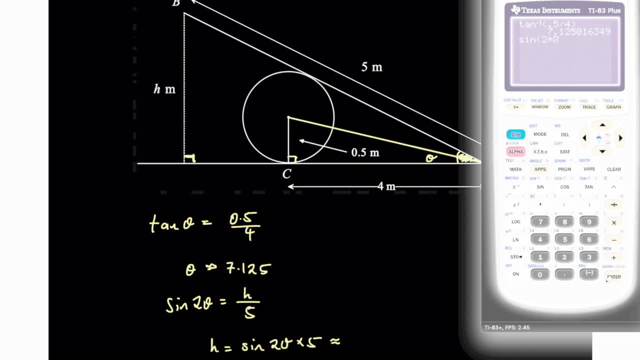 the previous answer. So I'll just do 2 times the answer and then multiply that by 5 and I get 1.2322 decimal place. So that's the right angle triangle. So now I can do the inverse tan of 2 theta. So I can do the inverse tan of 2 theta. So 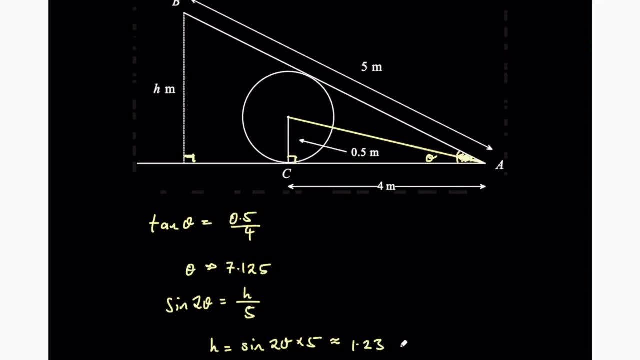 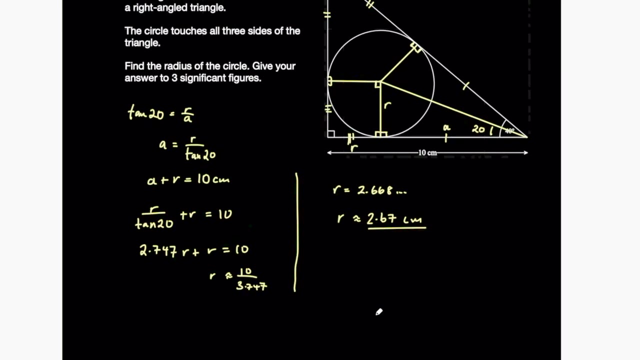 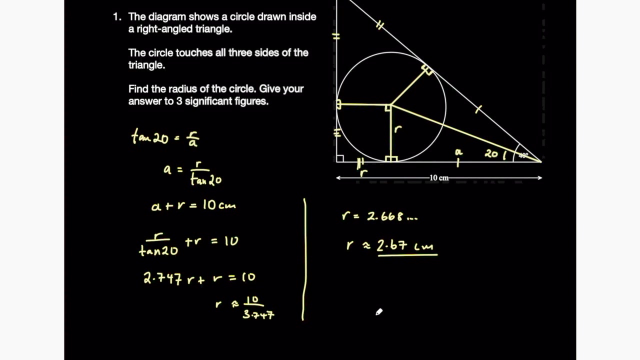 I'm going to do some ideas on how this is going to be okay and the first thing I'm going to then do is go into a similar problem and I can do the inverse tan of 2 theta and I can calculate that over a come, because obviously that's not a simple problem. 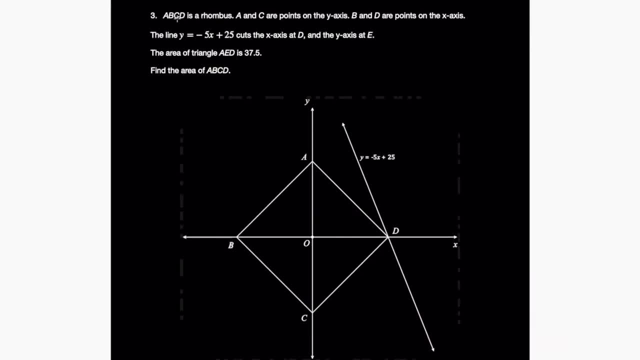 Yes, And, by the way, this is going to be the inverse tan of 2 theta multiplied by 5.これは on my YouTube. This problem says ABCD is a rhombus. A and C are points on the y-axis. B and D are 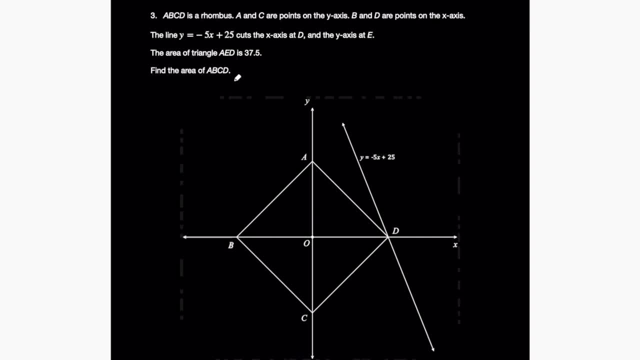 points. on the x-axis, The line y equals negative 5x plus 25. cuts the x-axis at D and the y-axis at E. The area of triangle AD is 37.5.. Find the area of ABCD Okay. so what do you need to find the? 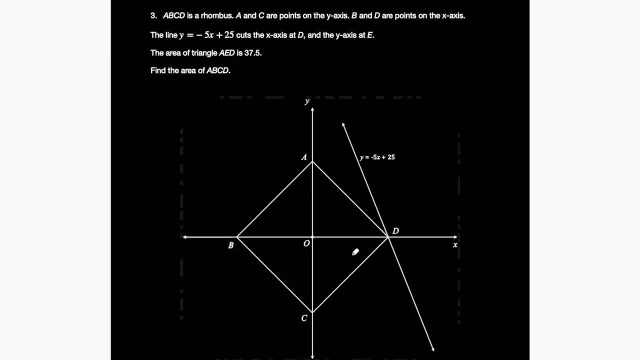 area of a rhombus. Well, it's the lengths of the diagonals. How could we know those? We could find the coordinates of these points A, D, C, B, And actually we only need two of the coordinates because we know that diagonals bisect in a rhombus. So if you find a point A, then you'll. 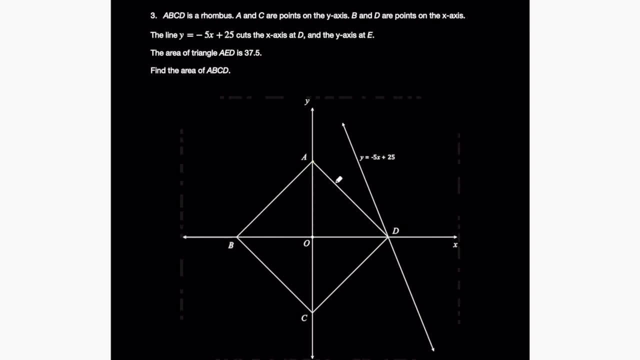 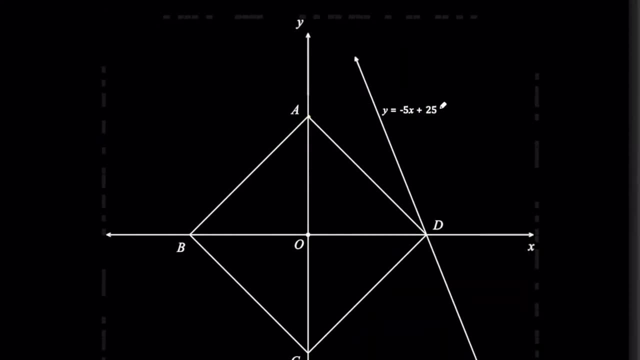 know point C. If you find point D, you'll know B. Okay, so let's focus on finding A and D. D we can find by using the equation of this line here, because they tell you the line cuts the x-axis at D. So then you can find point D by setting y equal to zero. 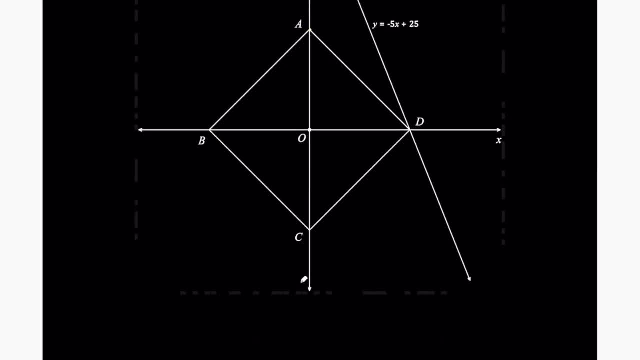 So, firstly, focusing on D, we can say that we'll have point D when y equals zero, So negative. 5x plus 25 equals zero. This will give you the x-coordinate. Well, what would x be here? It must be five, right? Negative 25 plus 25 equals zero, So x equals five, So we have point D. 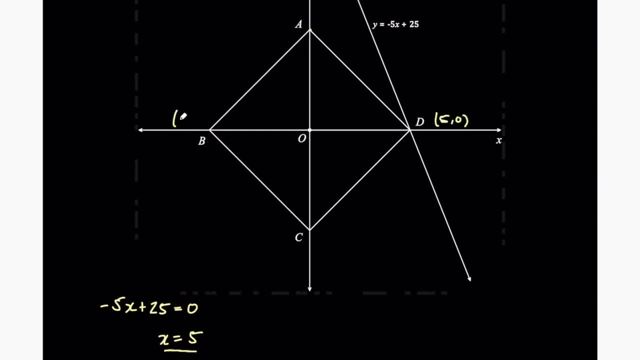 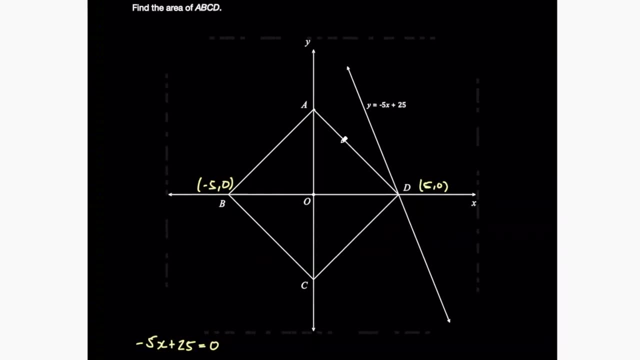 that's at five zero. Therefore, we also know B is at negative. five zero Must be the same distance from the center. And then we have point D. that's at five zero. So we have point D, Then we need point A. Well, this is where this area comes in useful, because they tell: 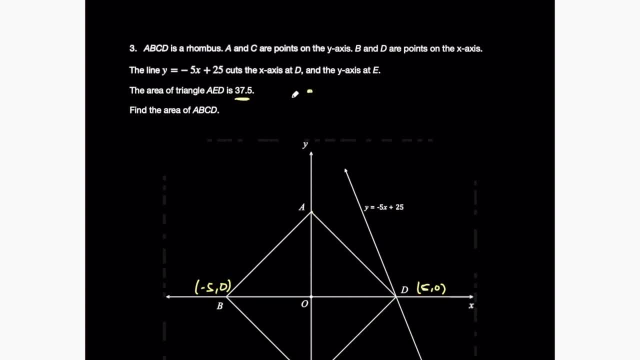 you. this line cuts the y-axis at E, So we need to find point E up here And you should know how to find the y-intercept of a line from the equation of that line. It's the constant added on the end. So looking at this equation, you should know that the y-intercept straight. 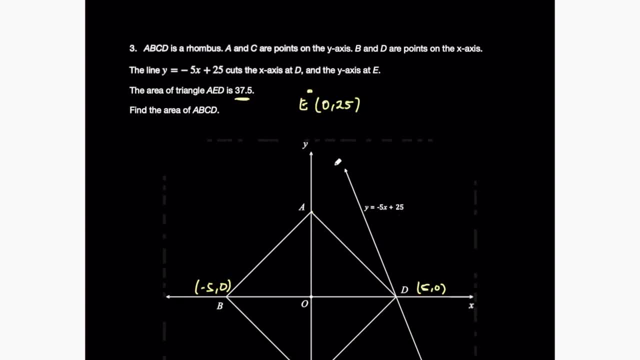 away is 0.25.. And then you need to think about compound shape. So if they tell you this area is AED, this triangle in here, if they tell you that area is 37.5, well, what does that mean? This area down here is OAD. Well, the height of this triangle is 25.. The base is 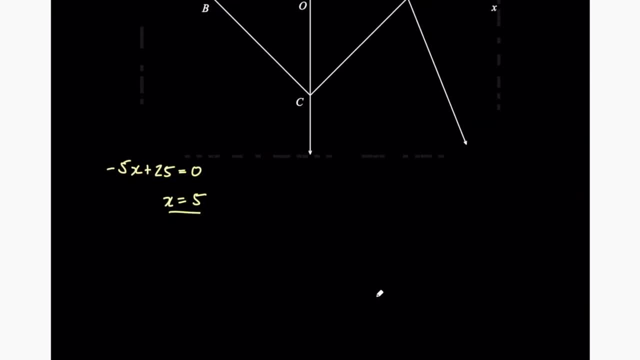 5. So let's write this down: The area of triangle OED, That's this big one. So let's write this down: The area of triangle OED, That's this big one. So let's write this down: The area of triangle OED, That's this big one. 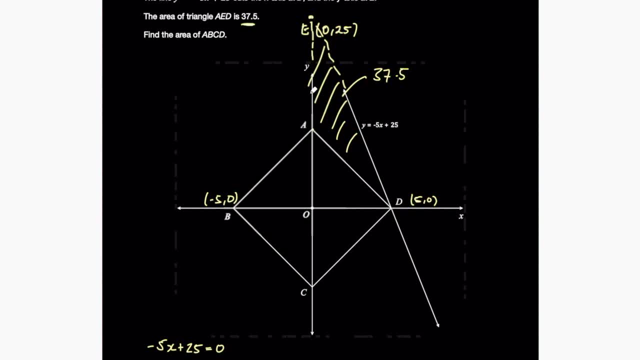 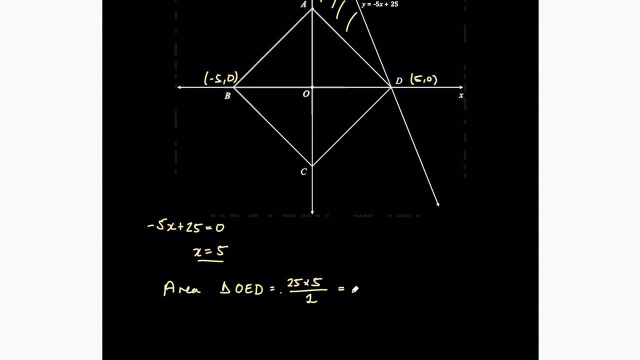 From O all the way up to E and down to D again, The height is 25.. The base is 5.. So this would be 25 times 5 divided by 2.. That's 125. divided by 2. That's 62.5.. Okay, So that's. 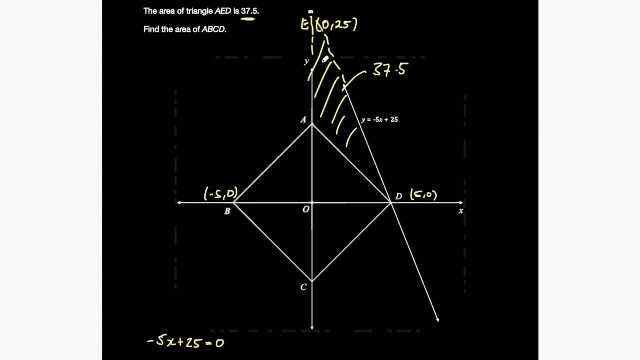 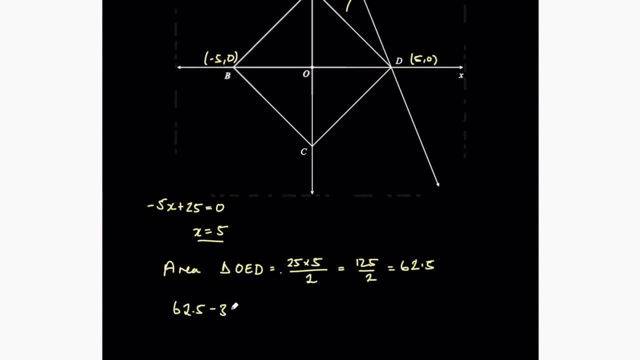 the large triangle OED, Then take away this area AED, which is 37.5.. Let's do 62.5, take 37.5. This would be the area of the triangle OAD. Okay, So triangle OAD, That's the area, Sorry. 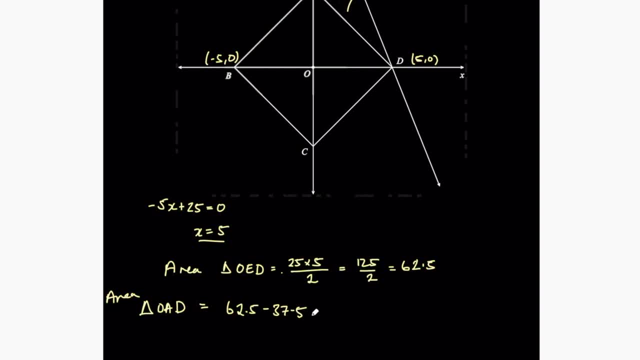 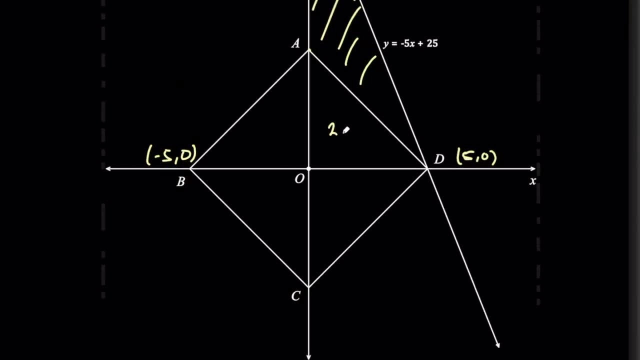 I'm messing this up a bit: 62.5, take 37.5. That's 25.. Okay, So this area in here is 25.. And actually you don't even need to use that area. You don't even need to use that area. 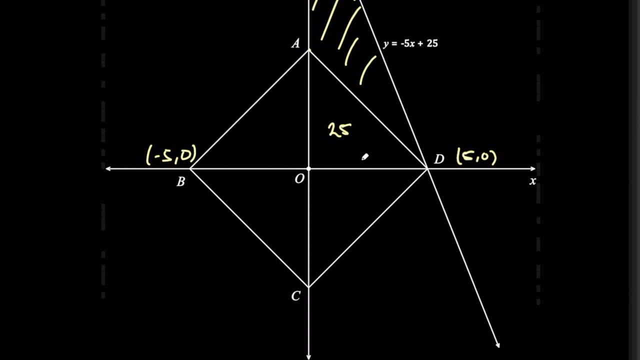 To find the coordinates of A, although you can, because if this base is 5, the length of the base here, OED, is 5, that must mean A is at a height of 10 or 0.10.. So 10 times.